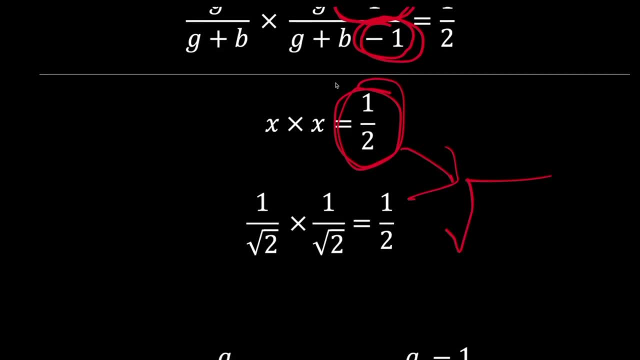 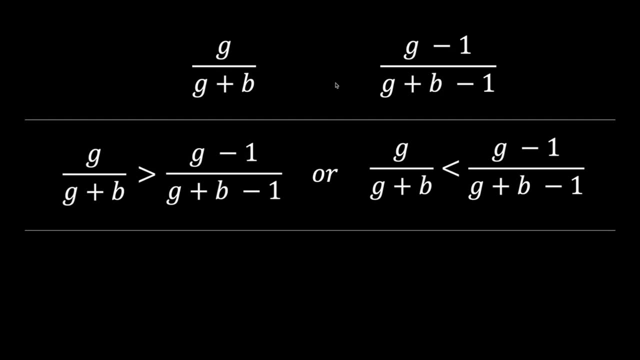 of 1 over 2, giving 1 over square root 2 for the value of x. But the two terms we have are different though, So which one is bigger, the left or the right? Given a proper fraction, since g and b are. 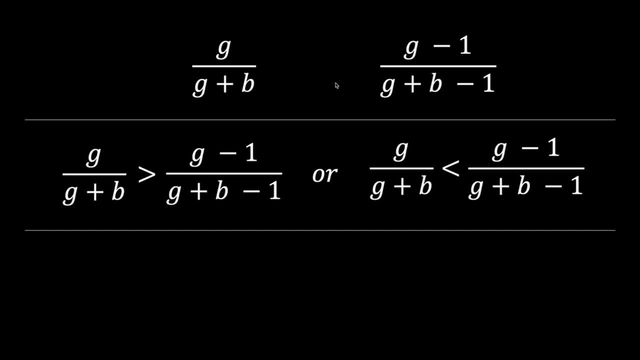 positive integers. what happens when we subtract 1 from the numerator and denominator- Starting from a toy example- 5 over 10, and subtracting 1 from the top and bottom? this results in smaller numbers. Hence the terms with the subtraction zone. 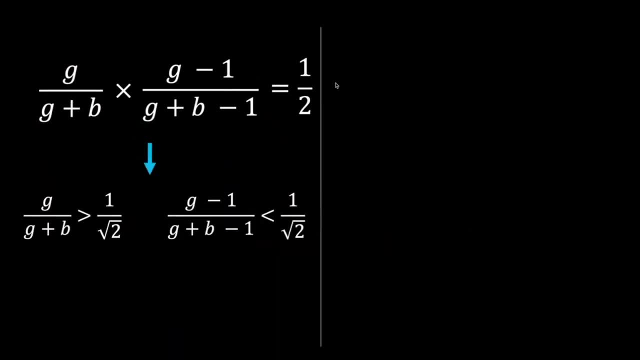 Knowing this, the following two inequalities are true. If this isn't clear enough, let's put together what we already know. Take two identical numbers, say 3, their product is 9.. But recall, we are working with two numbers that are very close to each other, but now one is larger. So let's 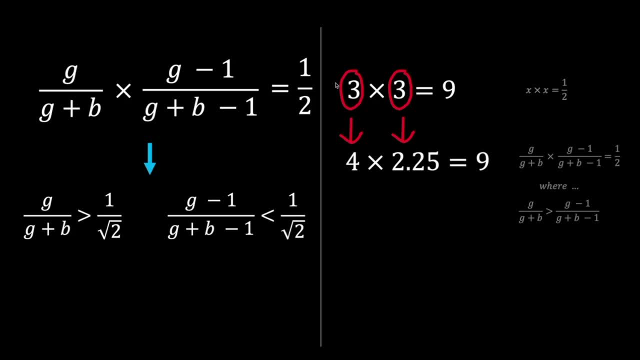 try that The first 3 is incremented to 4, the second term must then decrease below 3 to 2.25 for the equation to hold. It is obvious that 4 is larger than 3 and 2.25 is less than 3,. 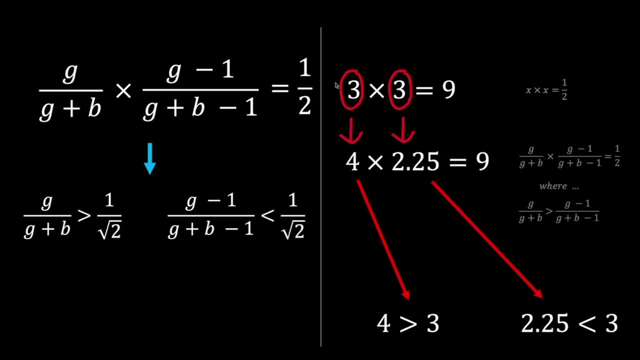 whereas 3 is the values of the product terms. if they were equal, Translating this back into our equation, the larger term must therefore be larger than 1 over square root 2, and the smaller less than 1 over square root 2.. Hence it now has some sense of. 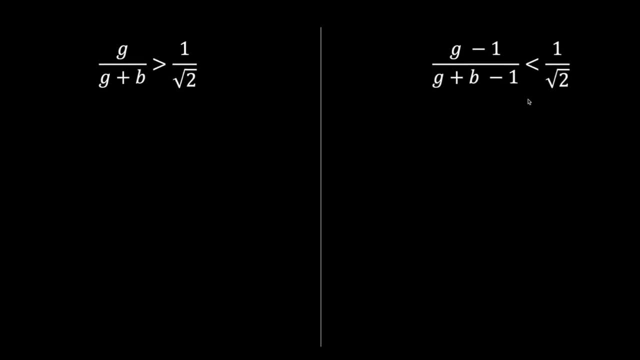 the range of values for our terms. With these two inequalities and after some trivial math, we obtain a range of values that bounds g. the number of green socks in terms of b, the number of blue socks. Putting these together, g's value is now bounded clearly in terms of b. 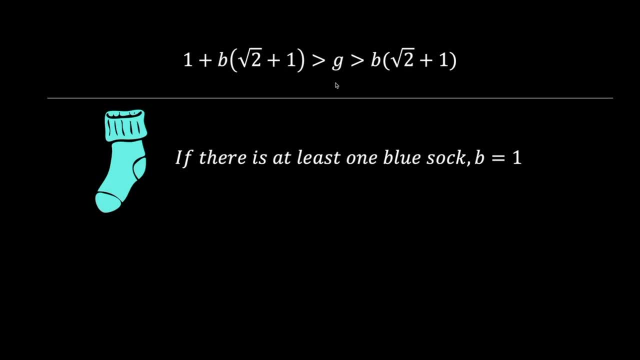 Since the problem requires at least one blue socket, which is the smallest possible value for the number of blue socks, let b equals to 1.. Plugging in the values, we see that g, an integer value, must be 3 when b is equal to 1.. As a sanity check, 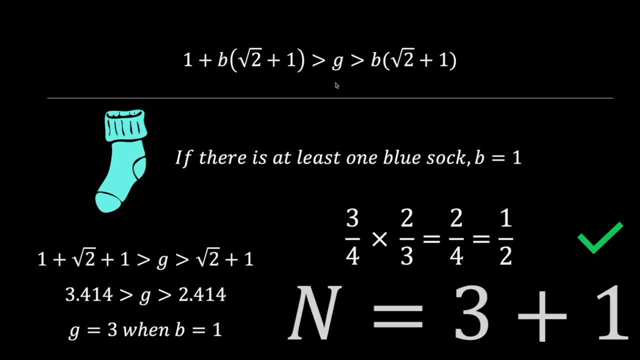 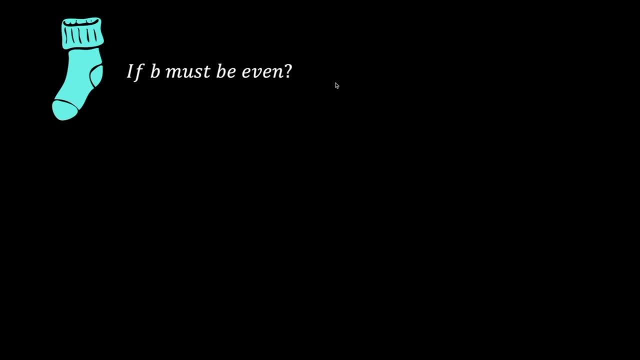 let's see if the probabilities hold, which they do. Hence n is equal to 3 plus 1, 4.. What if, instead, b must be an even number, So b can go from 2,, 4, 6,, etc. What is the smallest? 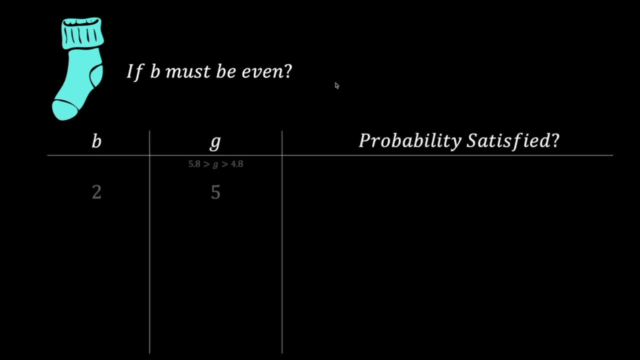 value of n. then Let's test that out. When there are two blue socks, by the inequality g is 5., Which unfortunately does not satisfy the probabilities. Similarly for 4 blue socks, However, at 6 blue socks with 15 green socks, the required probability is achieved. Hence